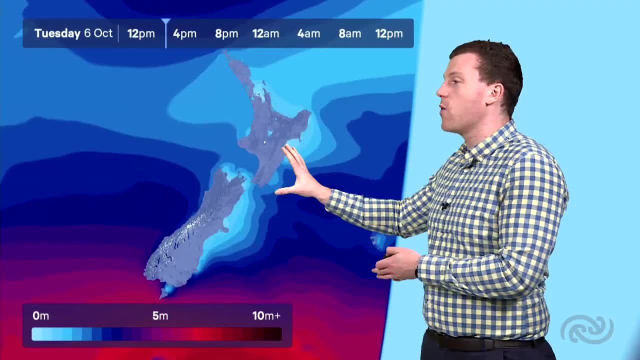 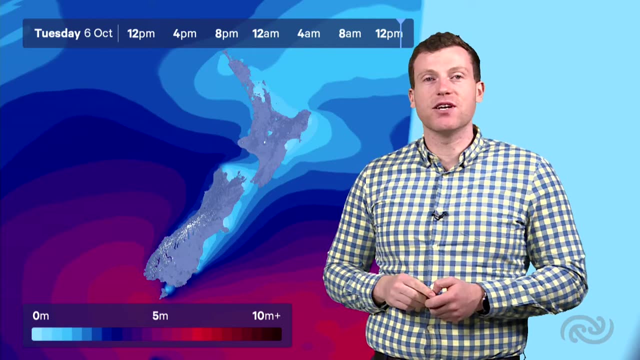 So you might have seen something like this before. This is a map of wave height, Swell height around the country, But this doesn't tell the full story. There's more to waves than just the height, And to show you that, we've got a little example here. 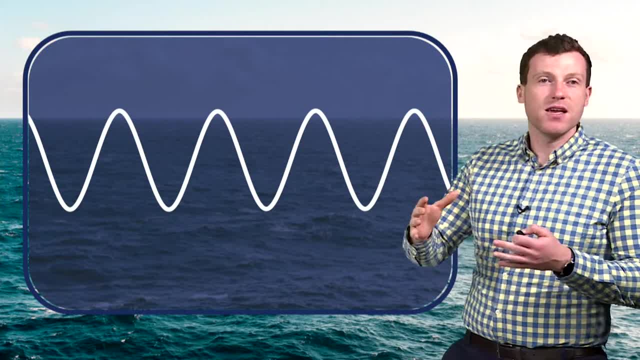 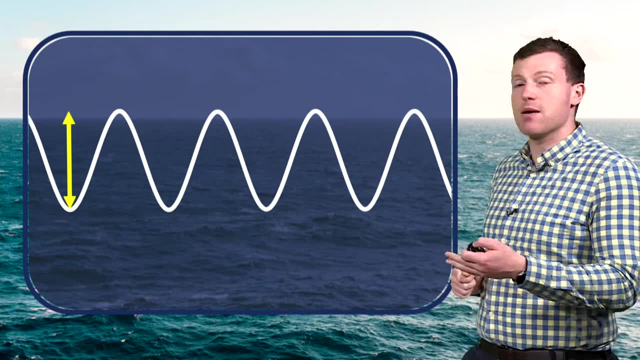 Now this is obviously very simplified Out. in the actual ocean the waves are much choppier. They're not as consistent as this, But the points I'm making all still stand out in the sea. What we just saw, the map before, was the wave height. 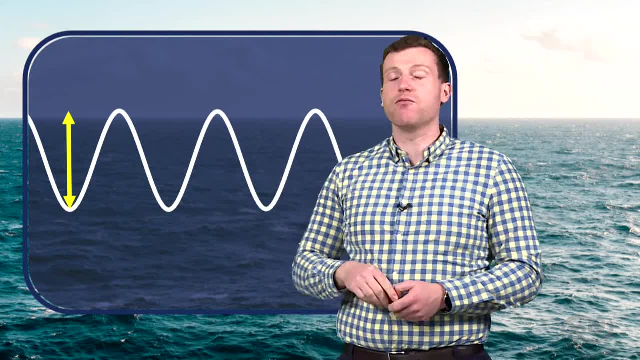 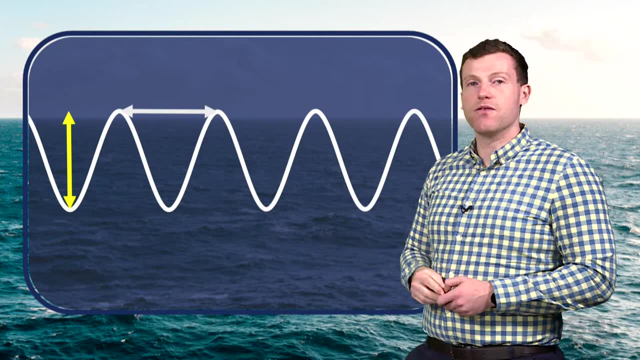 That is the distance between the crest and the trough of the wave, But there's more to a wave than that. This here is the wavelength. This is the distance between two successive crests of the wave, And these are not always the same. For example, here we have two different waves. 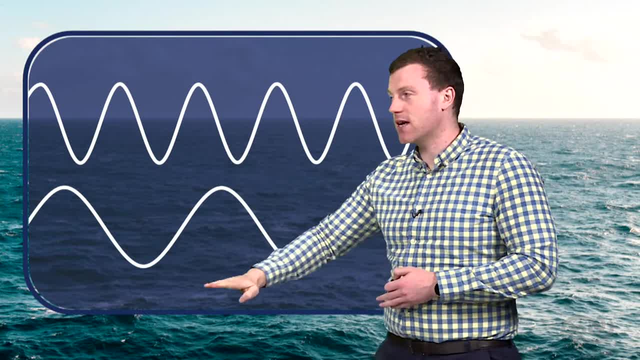 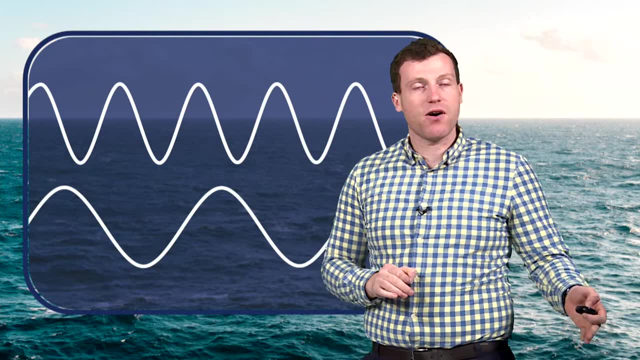 They have the same wave height, The same height between the crest and the trough of each successive wave. So these two wave schemes here would both come up looking exactly the same on the wave height map we were just looking at earlier, But clearly they have vastly different wavelengths. 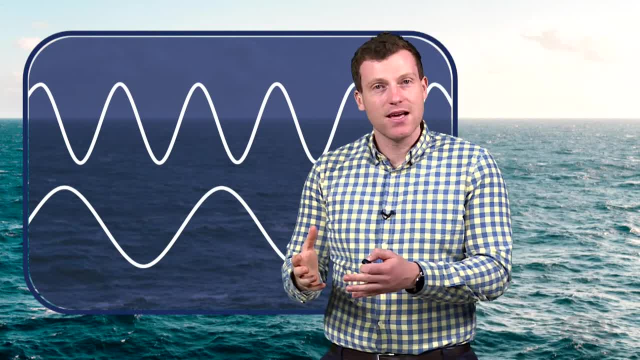 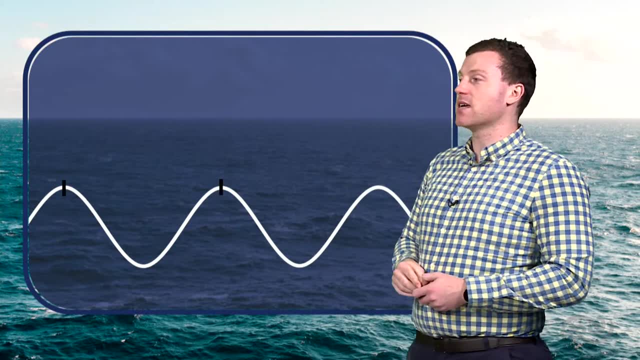 This one, in fact, is twice as long as this one. So the wavelength is what we're interested in, but that is not the same as the swell period. What is the swell period? Well, it's actually defined as the time taken for a wave to pass from crest to crest past a stationary point. 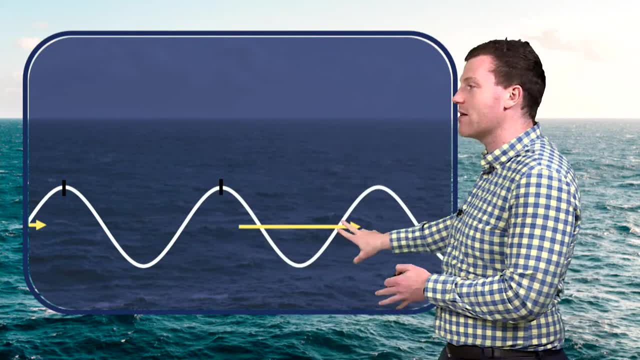 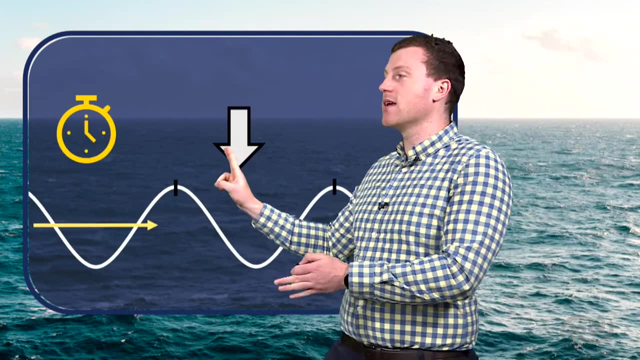 So you imagine a wave here. We've got two successive crests. This wave is in motion, We get a stationary point, We see the waves flying by and we time how long it takes between the first one and the second one. This is the swell period. It is related to the wavelength, but it is not the same thing. 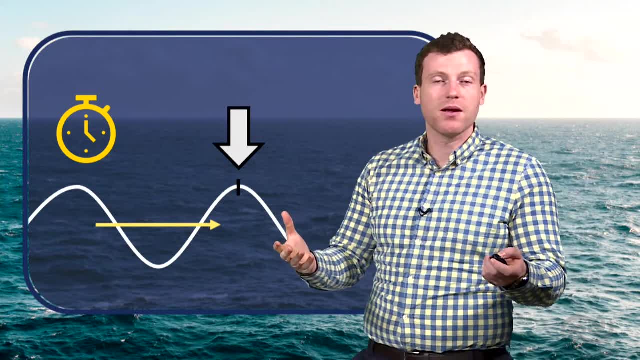 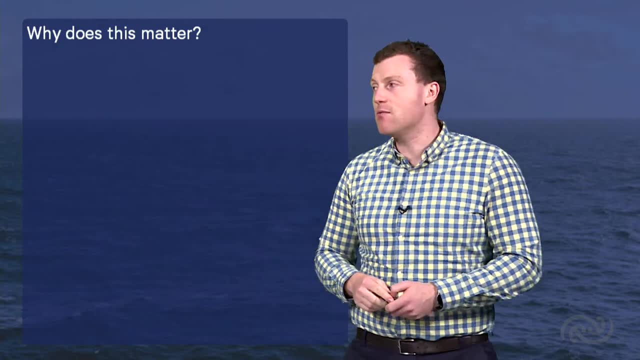 So we've started introducing swell periods Big deal. Why is that important? Well, it is important because waves of different period can have vastly different characteristics, even if they are the same height. In particular, the ones we're really focused on, the long period swells. 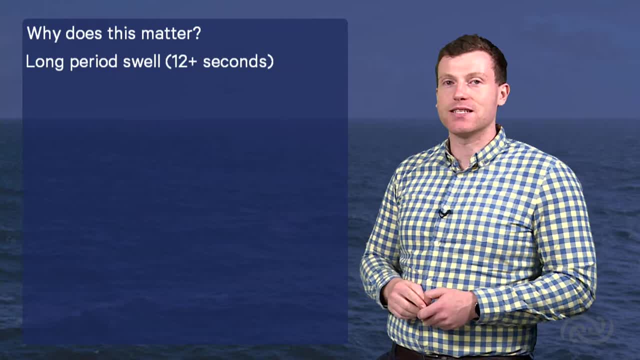 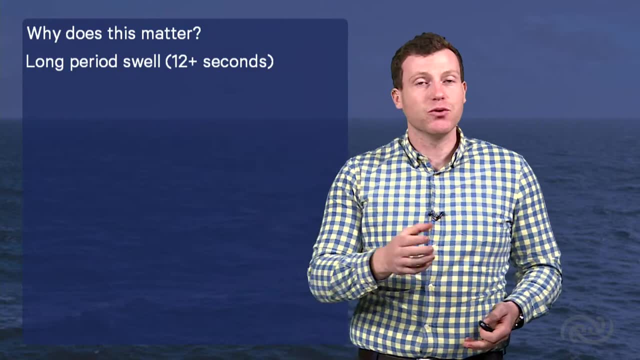 That's when we're seeing 12 or more seconds between each successive wave crest, And this number can get up pretty large. We can see 16 seconds, 18 seconds, In very rare cases up to 20 seconds between each passing wave.